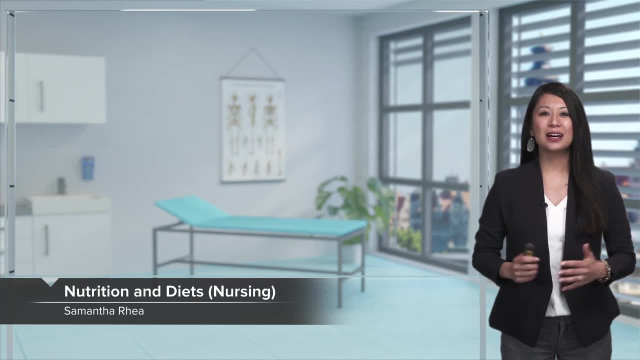 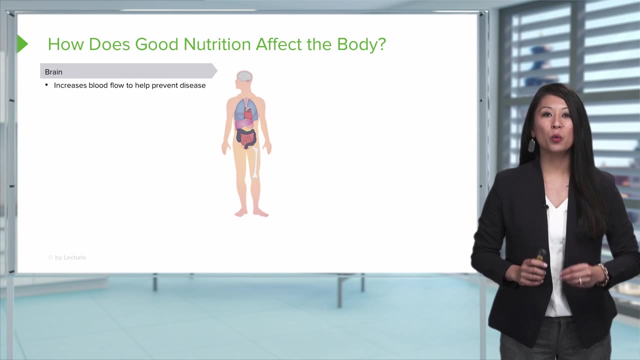 Welcome to the topic of nutrition. We're going to discuss about all of the positive aspects that nutrition can bring to your client, and also different types of diets and consistencies that you need to consider in regards to treatment of your patient. Now let's start off by talking about what good nutrition does to affect the body. Well, first off, 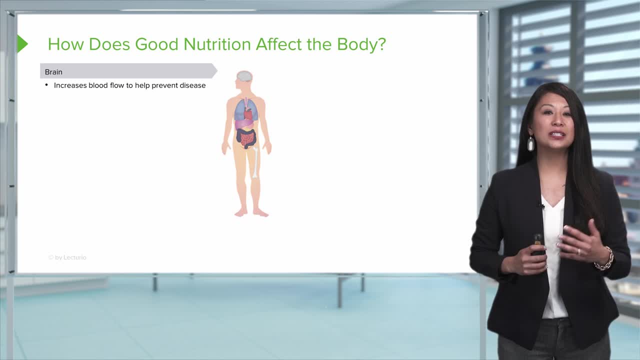 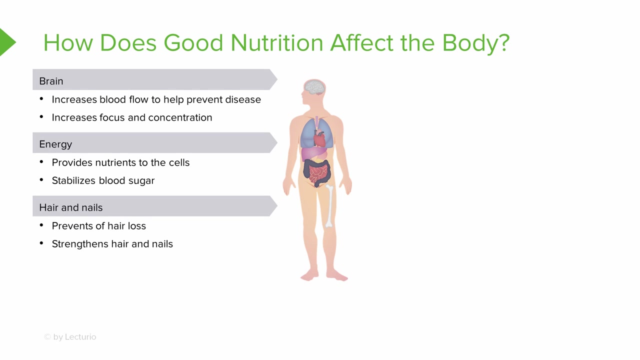 it helps increase blood flow to prevent disease, helps increases blood flow to our brain, increases that focus and concentration and, of course, provides great nutrients to the cells to provide great energy and help stabilize our blood sugar. Now don't forget about the advantages for good. 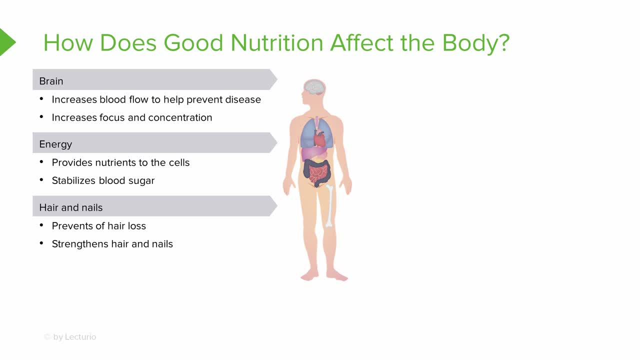 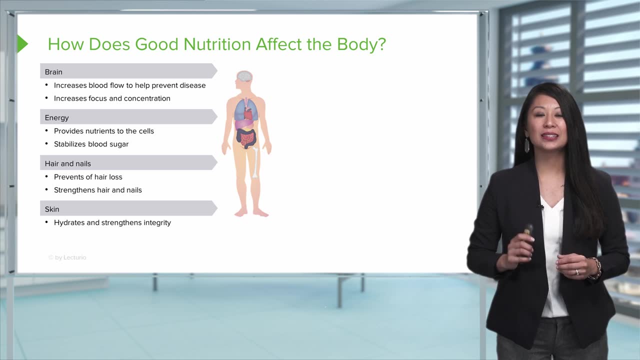 hair and nails. It can help strengthen those and prevent hair loss as well. And a really important point is: good nutrition can help hydrate and strengthen the condition and the integrity of the skin. Now, many of you know who are in nursing school or who are nurses, that 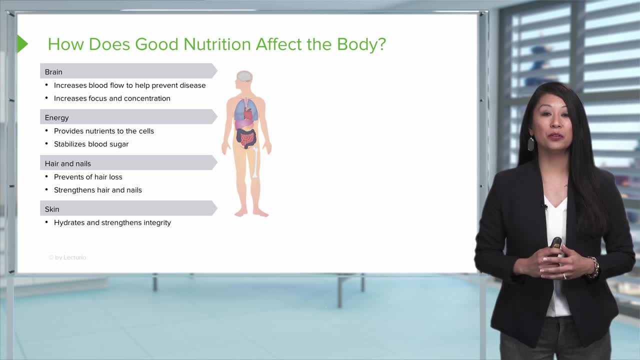 good nutrition helps prevent those wounds or even helps heal them. in that process It also can help prevent acne and infections. Now good nutrition really plays a key role in immunity to help boost that, to help prevent disease prevention, Not to mention that it'll help again. keyword: good, healthy nutrition reduces fat and cholesterol to decrease heart disease. 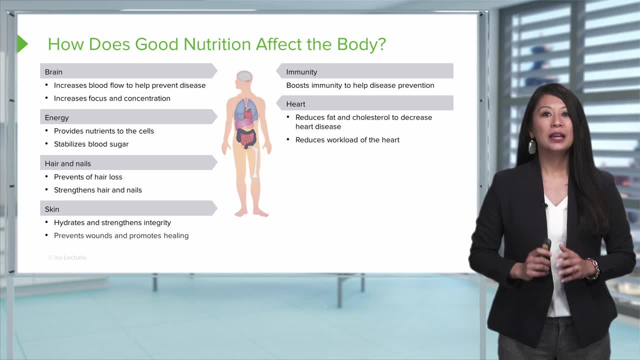 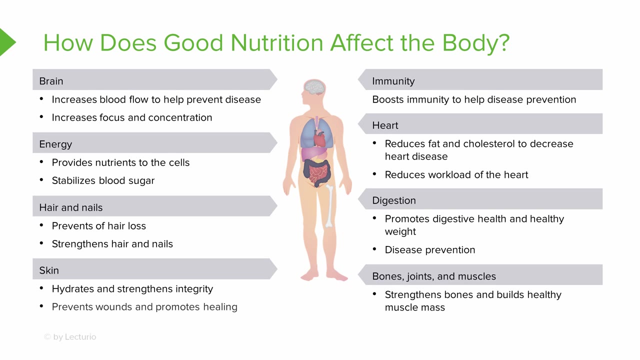 and reduce the workload of the heart. Now, digestion is another thing we've got to think about. in regards to good nutrition, It can help promote good digestive health, healthy weight and disease prevention. Now, lastly, good nutrition is key for good bones, joints and muscles, To strengthen those build. 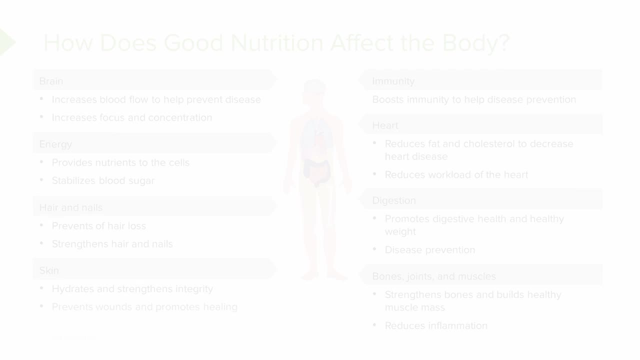 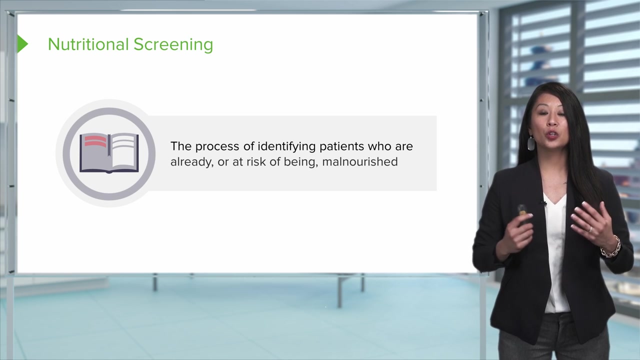 healthy muscle mass and reduce inflammation. Now let's talk about nutritional screening. This is commonly done in many different facilities for our clients to assess what their dietary. Now this is the process of identifying patients who are already or at risk for malnourishment. 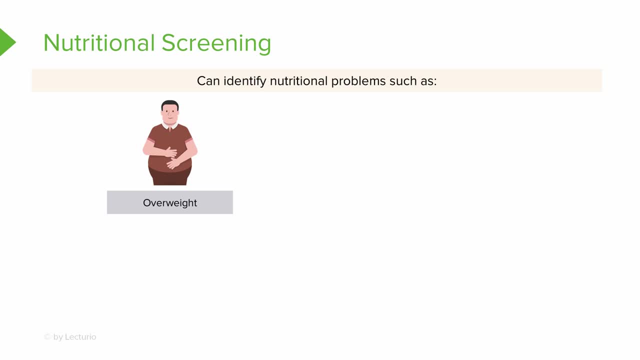 A good nutritional screening can identify many different problems, such as being overweight, underweight, if there's a significant weight loss or gain, poor food choices, social habits- that can affect our nutrition. Now the availability of food is another key piece and any potential problems with digestion that you may have. 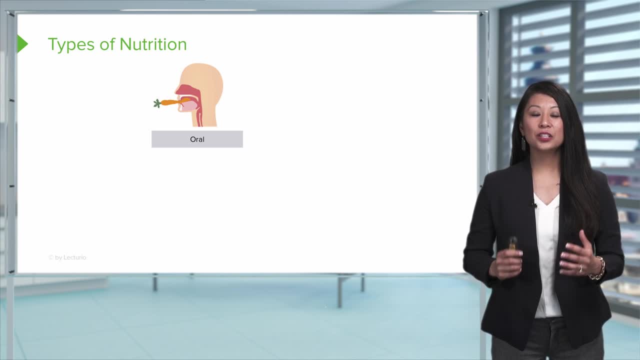 Now let's take a look at different types of nutrition. As a nurse, there's different routes that sometimes we need to use to help maintain our patient's caloric or dietary needs. Now, the first is the oral type of nutrition, which, of course, is the most preferred, and this is by just taking food. 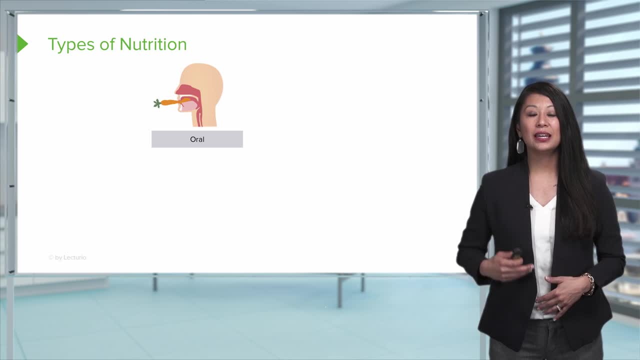 or supplements by mouth down the esophagus into the digestive system to get that good painkiller and the oral type of nutrition which of course is the most preferred. And this is by just taking food or supplements by mouth down the esophagus into the digestive system. 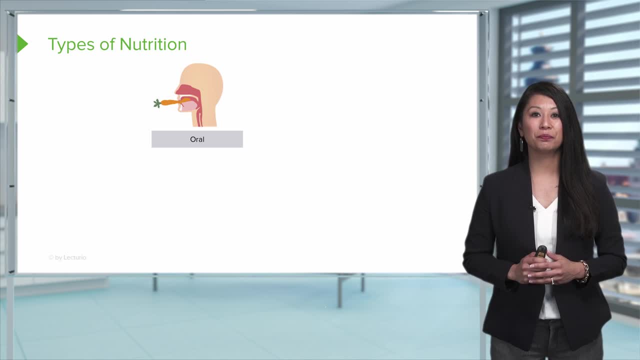 peristalsis, which is the most ideal for consumption. Now, sometimes for oral consumption, we may need some supplementation to help maybe increase protein or calories for our clients, and supplements can be used for specialized dietary needs. Now there are several instances where maybe the patient can't use the most preferred route, such as oral nutrition. Here's: 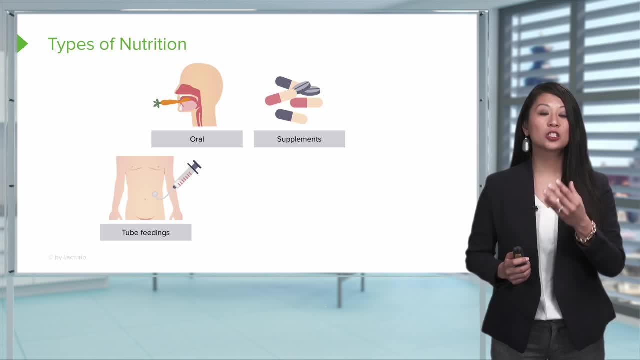 a great example of this. Maybe a patient, for example, can't swallow effectively, going into the patient's lungs which they can aspirate. Of course, this is a patient safety issue and dangerous. Therefore, sometimes we have to bypass the oral route and go, for example, using tube. 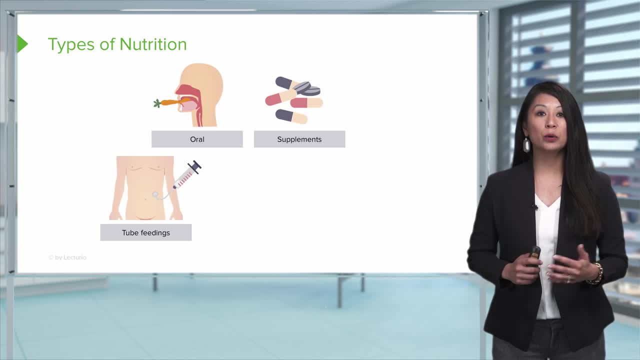 feedings. Now we can support their nutrition using liquid feedings that supply directly to the gastric region through, maybe, the nasogastric tube, an oral gastric tube, or a PEG tube which goes directly into the stomach. Now we can also use IV fluids to help. 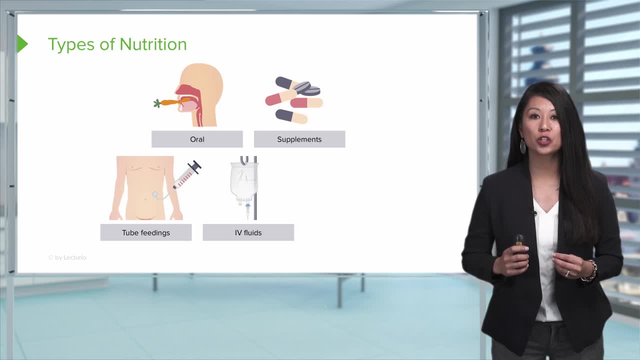 support, hydration and electrolytes. but again, this is more of a short-term therapy. And don't forget, we also have something called TPN, otherwise known as total parenteral nutrition. Now, this is a little bit longer term than IV fluids. It's nutritional therapy that has lipids also for 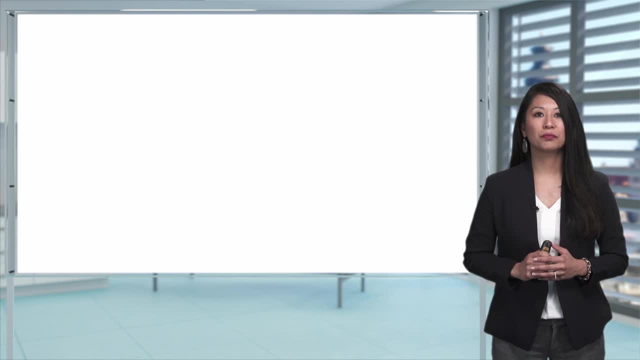 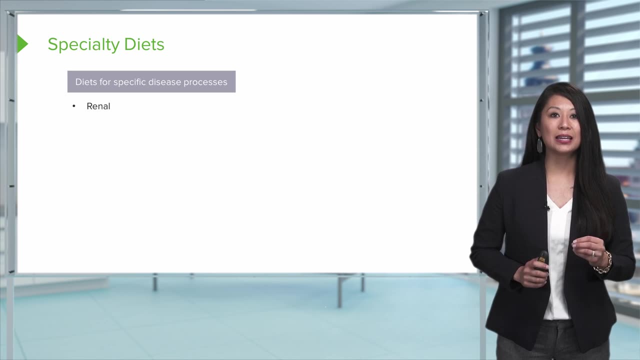 energy, different hydration electrolytes. Now let's take a look at some specialized diets. We'll just talk about these briefly. Note that there's special diets for specific disease processes. For example, there's a renal diet if a patient has kidney disease, A diabetic diet for diabetics. of course, There's low sodium. 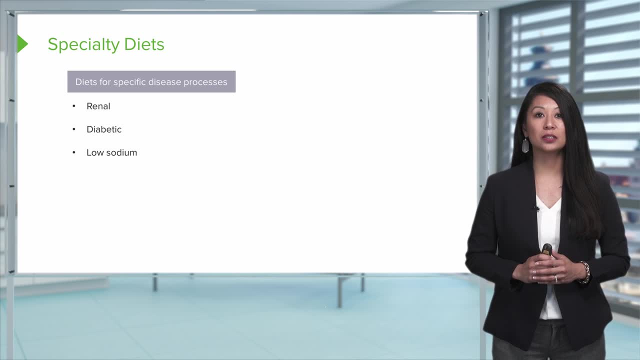 diets that we use many times for cardiac patients And, of course, if your patient's malnourished. sometimes we may need a high calorie or a high protein diet. Also, if a patient has delayed wound healing, we may also use a high-calorie or high-protein. 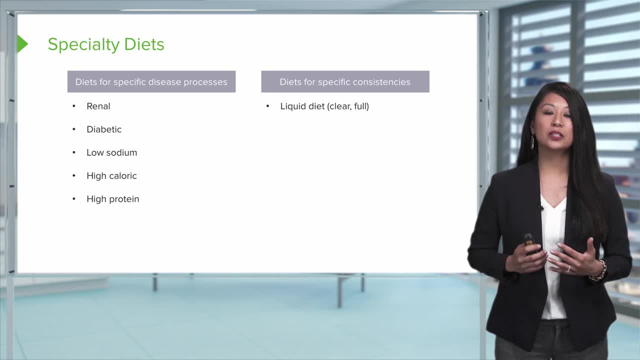 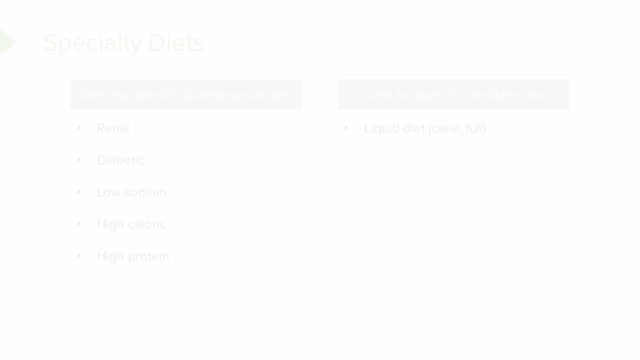 diet Now, due to swallowing difficulties or maybe the patient's preparing for surgery. there are certain diets for specific consistencies, such as a liquid diet, which also, if the patient has any inflammatory bowel issues, for example, we may use that type of diet. 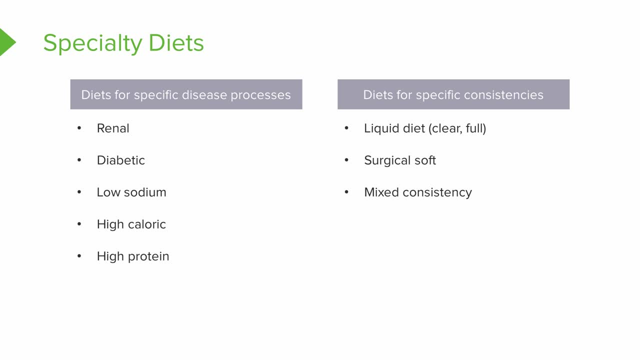 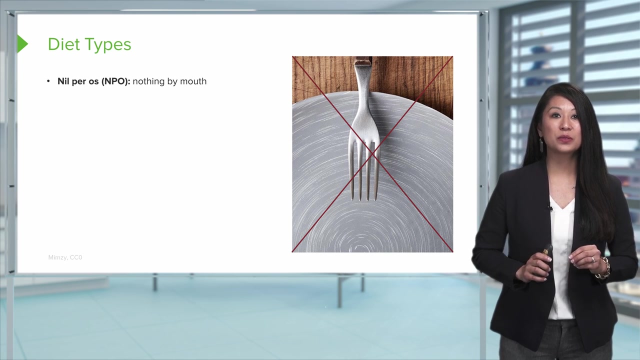 There's surgical soft diets, mixed consistencies. Sometimes we may need to ground up the patient's food for swallowing, We may need to even chop up the food- and, of course, there's a regular consistency diet. Now let's talk about some specific diet types. 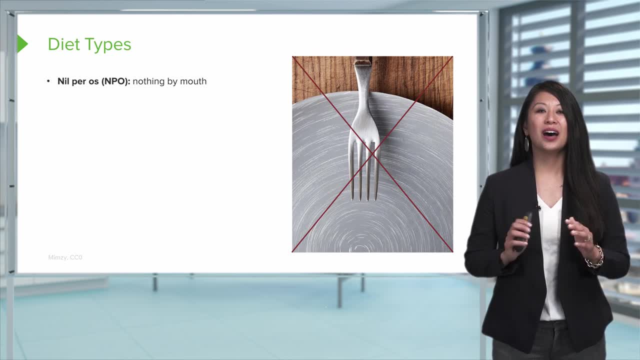 NPO is one that you're going to commonly hear as a nurse, otherwise known as nothing by mouth. This absolutely means we don't want anything to eat or drink down the patient's oral route. Now, just be conscious as a nurse, because sometimes the physicians 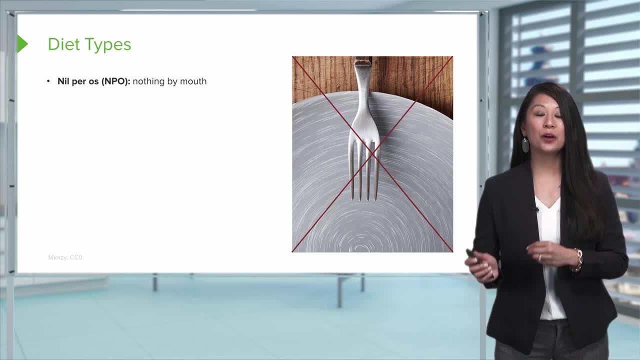 may be saying NPO or nothing by mouth, except for meds. So if you're going to give medications and you see the order for NPO, make sure you look at the order and clarify. Next, don't forget there's a clear liquid diet. 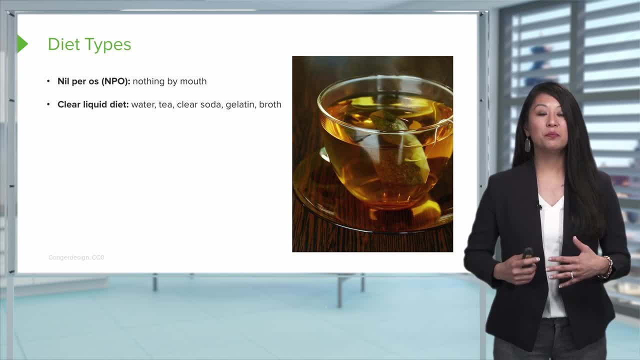 This is really helpful after the patient's been NPO- then maybe they're arousing from anesthesia. We may use that type of diet so the patient doesn't get nauseated. This can include water, tea, clear soda. You may want to include, of course, an anticoagulant. 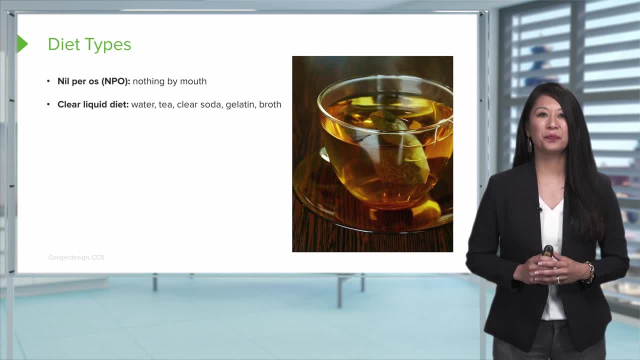 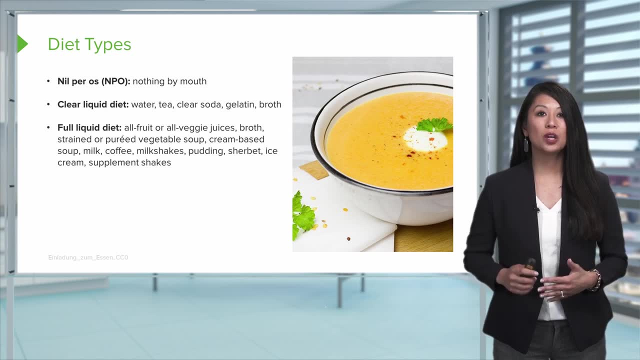 And so it varies depending on the individual. 葦, even gelatin, think about. it's kind of clear or broth. Now, if the patient tolerates that, especially post-surgery, or if they've had any gastric issues, we can then advance them to a 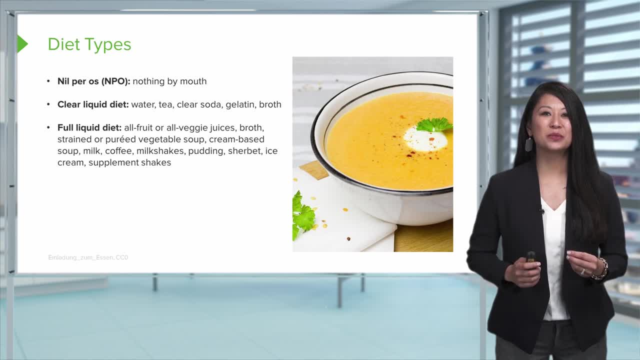 full liquid diet. Now, this is going to have a little bit more substance to it, a little bit more calories, but still very easily digestible. So this is going to include things like fruit or veggie juices, some broth. We can even use strained pureed vegetable soups, cream-based. 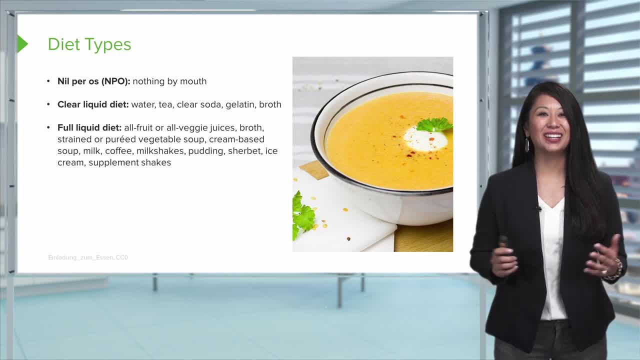 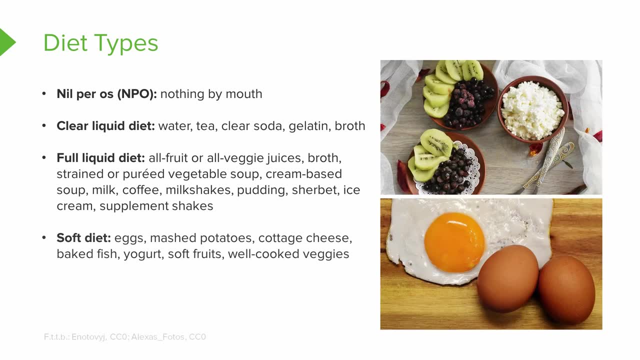 soups, milk, coffee, milkshakes, pudding, all some of those good stuff. Don't forget as well that if they can tolerate the full liquid diet, we can also use like a soft diet- Again still easily digestible, but got a little bit more bulk to it, So this can include something like eggs or mashed.